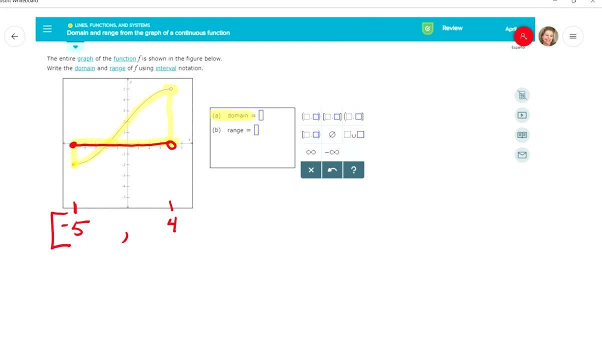 where the 4 is. that means you get as close to 4 as possible, but don't include 4.. And getting as close to 4 as possible would be 3.9999999999999999999999999999999999999999999999999999999999999999999999999999999999999999999999999999999999999999999999999999999999999999999999999999999999999999999999999999999999999999999999999999999999999999999999999999999999999999999999999999999999999999999999999999999999999999999999999999999999999999999999999999999999999999999999999999999999999999999999999999999999999999999999999999999999999999999999999999999999999999. 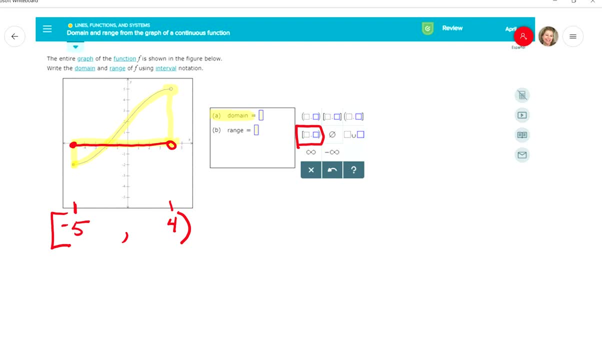 starts with a bracket and ends with a parentheses. So I'm going to click on that, so it'll go into this box, and then I'll just type in the negative five in the first box and the four in the second and that's my domain, The range. I'm going to erase this so I can do range next. 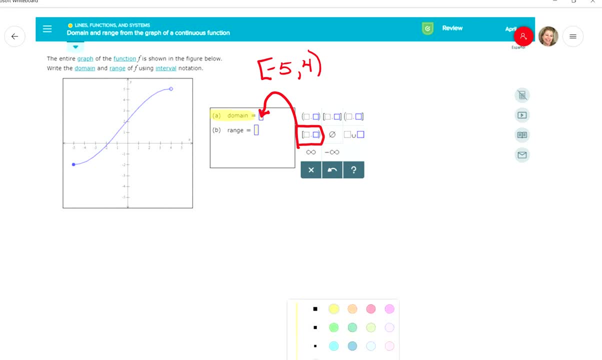 Um, the range covers your y-axis, All right, so I'm still looking at this same function, but now, instead of looking at it from left to right, which is how the x-axis goes, I have to look at it from bottom to top. So the bottom most point is still this one. This one is the far left point, but it's. also the far most point, So I'm going to click on that one. I'm going to click the bottom most point, and then I'm going to click on the right. So I'm going to click on the left, So I'm going to click the. 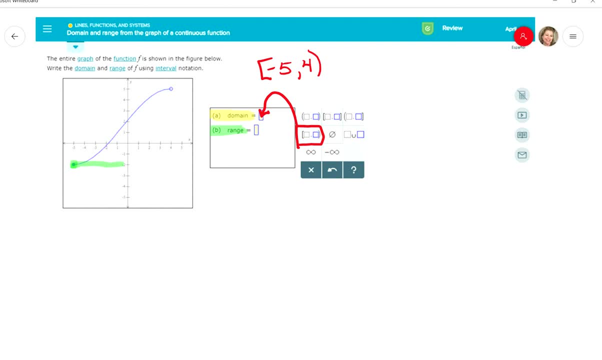 the bottom most point and that is at negative two on the y-axis and then as you go up the function you end here. so this is my highest and that one. the highest point is at five. so everything in between here on the y-axis is my range. so for this one it starts here and then goes all the way up to the five. so 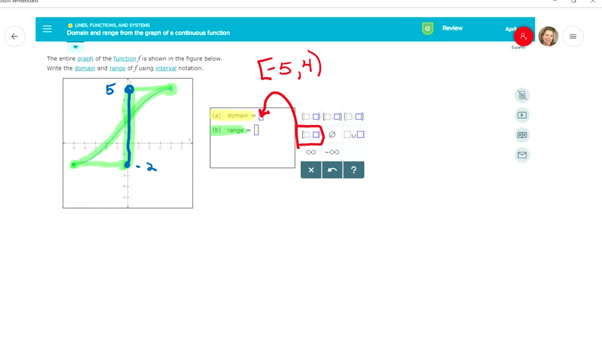 this was negative two, and up here is five and your interval. once again, it starts with a solid dot and ends with an open circle, so I'd need this same one to go in here and in there. I'm going to type the negative two And then the positive 5.. 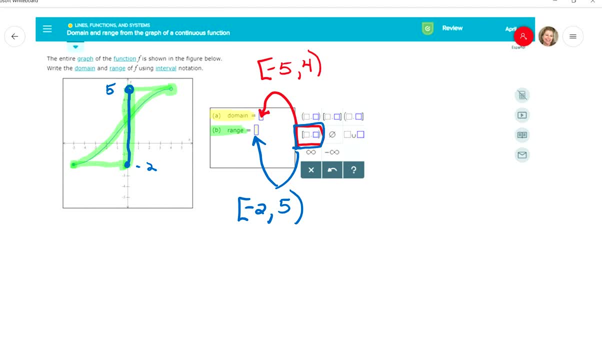 Intervals always go from smallest to largest. So for the domain, you're going to be going from left to right, Left to right, And for the range, you'll be looking at this thing from bottom to top. All right, So my x-axis was from left to right. 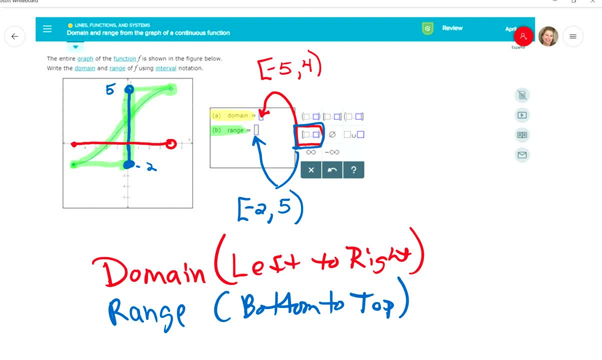 That's my domain. My y-axis was from bottom up to top. So every single point that's on this function. I'm going to click on Eraser again so I can show you something, Any point, Any point that you pick on this function. let's say we pick this point right here. 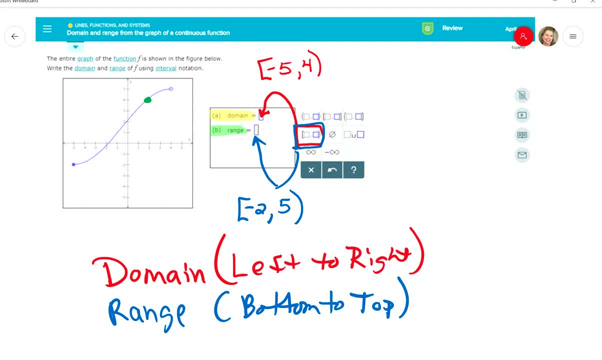 Okay, It has an x-coordinate, that's: let's say, it looks like 2.. And then it has a y-coordinate, that's 4.. So this ordered pair is the point 2, 4.. However, the x-coordinate of 2, 2 falls somewhere between negative 5 and 4.. 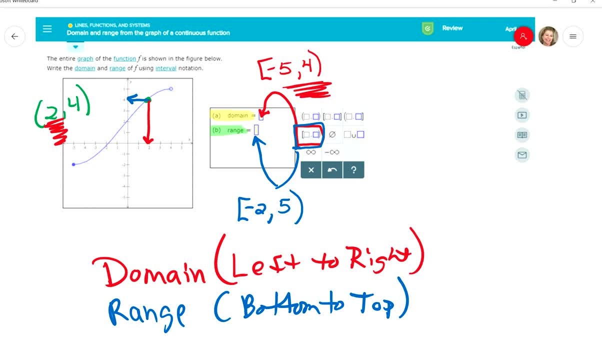 It's in that domain. And then the y-coordinate of 4, that falls somewhere between negative 2 and 5.. 4 is between negative 2 and 5. Just like the 2 is between the negative 5 and 4.. 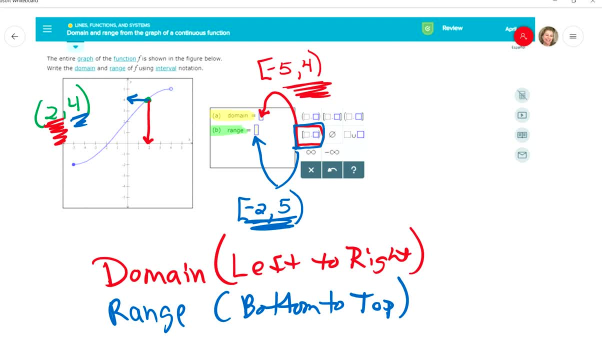 And I can do that with any point. Any point I look at, Its x-coordinate will be somewhere in this range and its y-coordinate will be somewhere in this range, Although they call this one up here the domain. Sorry, This one's the domain.